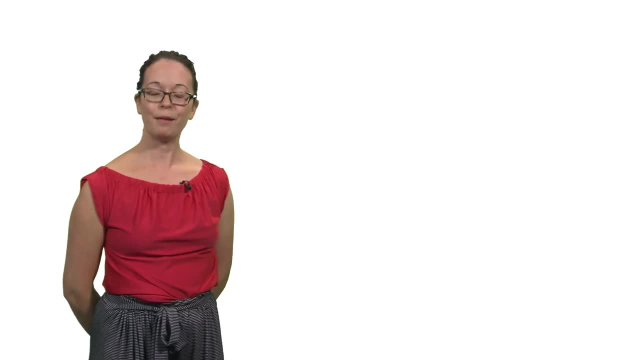 Hi, my name's Lindsay Leach and we're going to be talking today about the null and alternative hypotheses. So the null hypothesis is something that we believe or expect to be true. So, for example, we know that bees make honey, but this knowledge could stand trial against an. 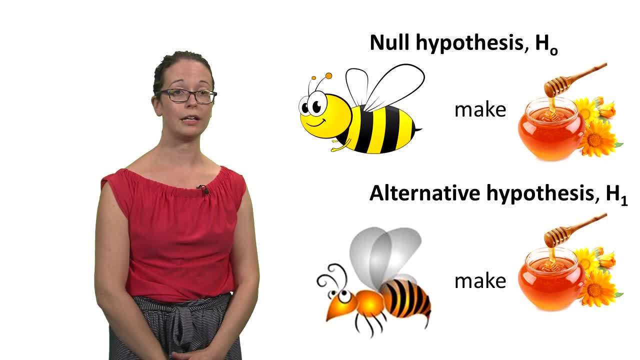 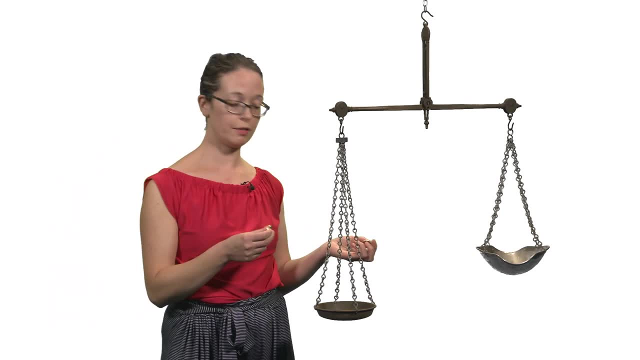 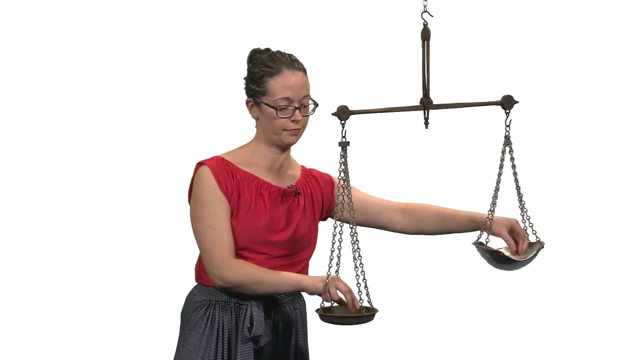 alternative counter claim. For example, wasps make honey and we call this the alternative hypothesis. Now let's imagine we have some evidence for each of the null and the alternative hypotheses: Here on the left, the null hypothesis and here on the right, the alternative hypothesis. 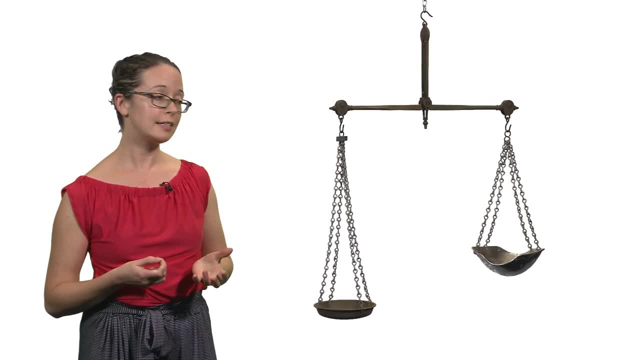 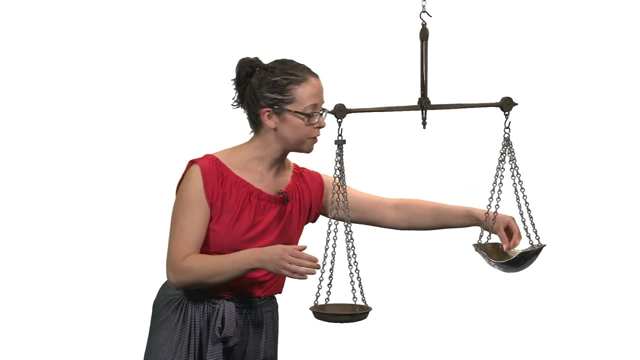 Now we have to assume that the null hypothesis is true unless it can be proven to be wrong. So as we start to sample from the population of interest, it may be that the weight of evidence starts to fall in favour of the alternative hypothesis, and increasingly so until we accept. 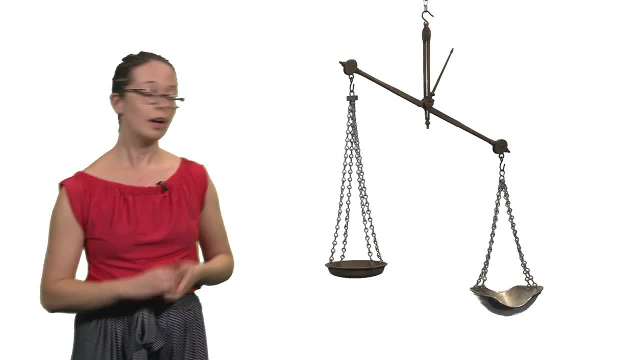 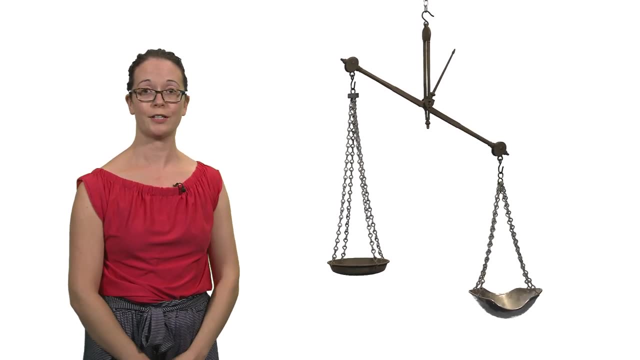 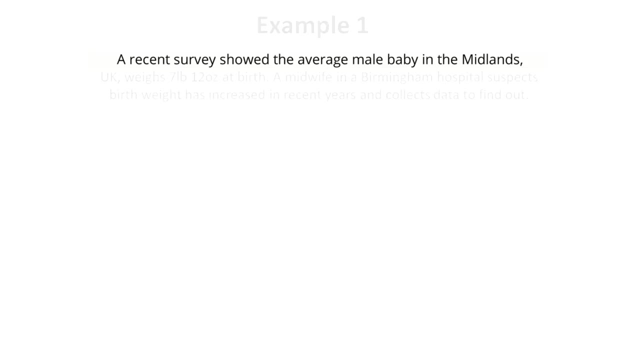 this new knowledge as truth. But if we accept the alternative hypothesis, we have to reject the null hypothesis, and the same would be true in reverse. To define what our null and alternative hypotheses are, we need to think carefully about the question. Here's an example. So in this example, we have a survey which showed that the average 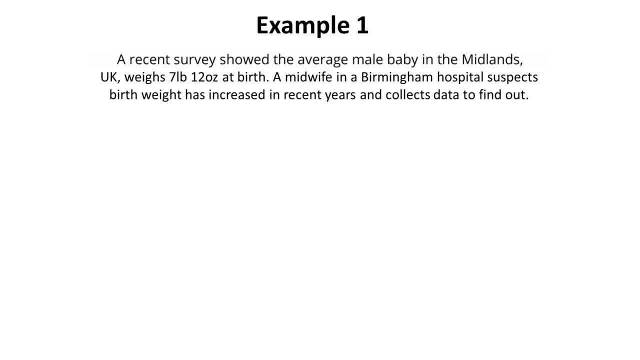 male baby in the UK weighs seven pound twelve ounces at birth, but a midwife in a Birmingham hospital suspects that the birth weight may have increased in recent years and collects some data to find out. So, as we said before, the null hypothesis is what you would expect to see, So based 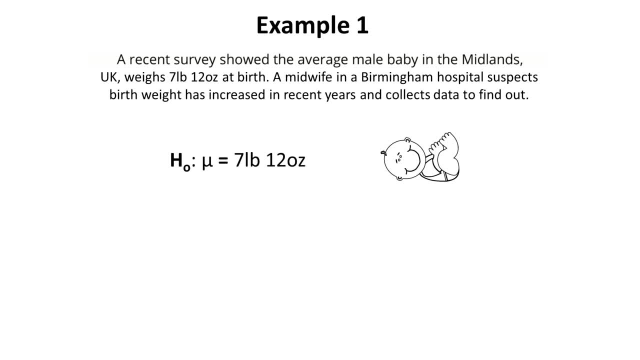 on the survey, we would expect that the average birth weight in the population, the mean mu, is equal to seven pound twelve. So that defines your null hypothesis. The alternative hypothesis is the new idea. So in this case the midwife believes that. 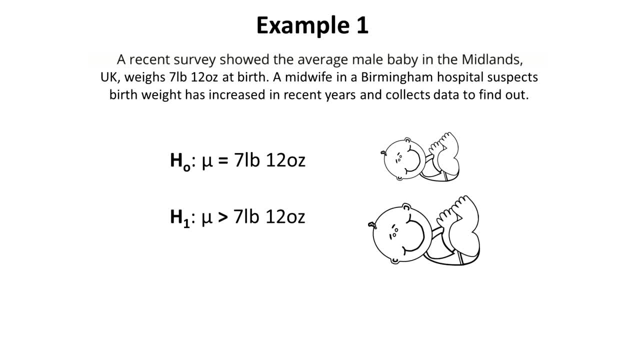 the birth weight has increased in recent years, So the alternative hypothesis mu is greater than seven pound twelve. So we could have used a range of alternative symbols here, depending on what the midwife wanted to test, For example less than, less than or equal.